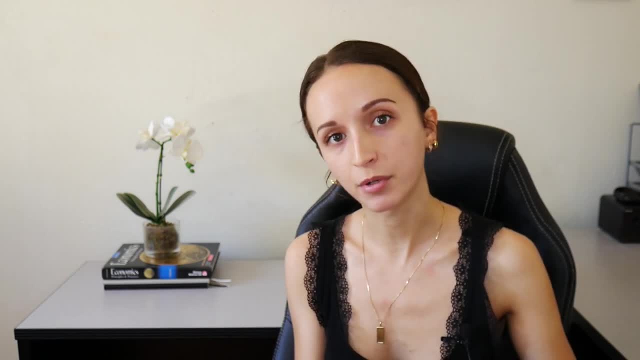 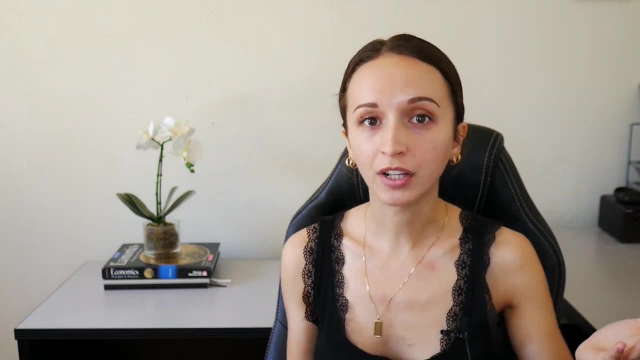 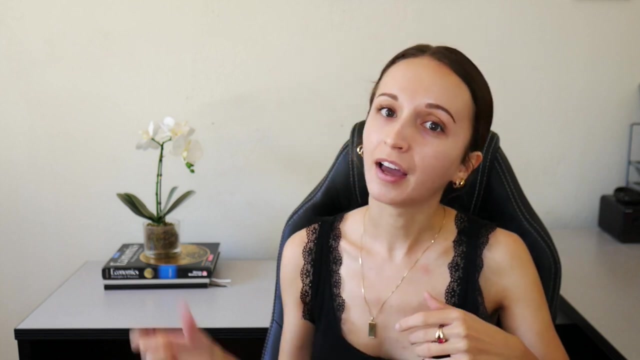 Define it from an economical and real life perspective and then explain how you can apply it to your personal life. Let's get into it. Also, if you enjoy learning new, innovative ways to navigate this crazy, crazy life, like and subscribe to this teeny tiny YouTuber and let's get a move. 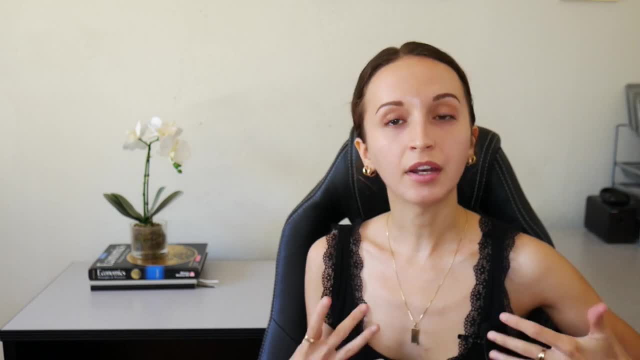 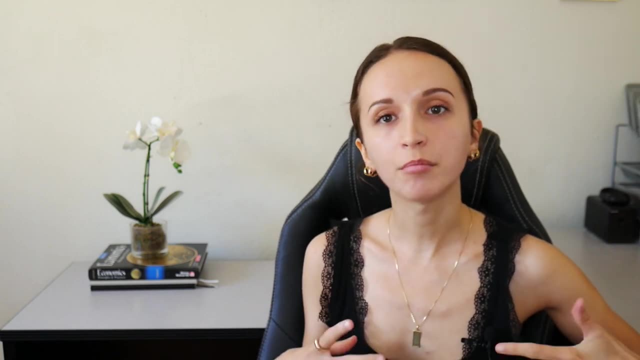 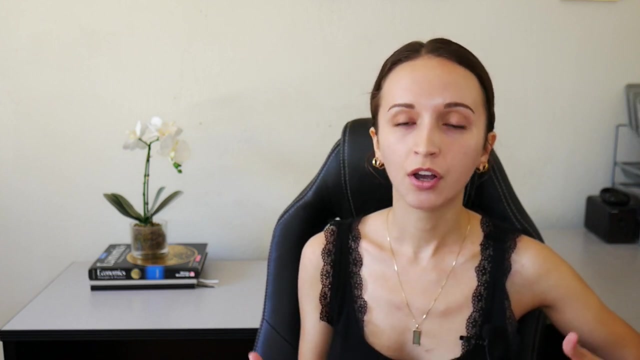 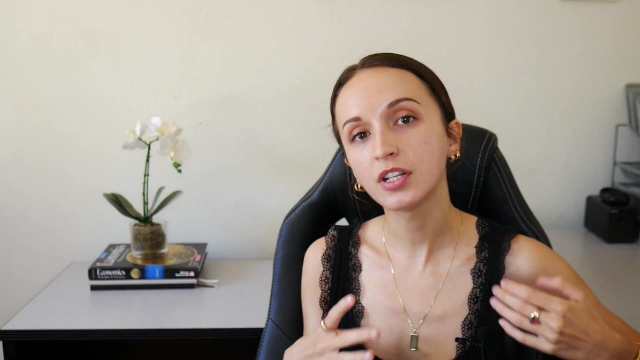 on Now in economic decision making. sunk cost refers to an investment that has already been made that cannot be recovered. These costs can refer not only to money, but also your time and your energy, Although money usually is the biggest motivator. Here's the kicker with sunk costs: When businesses decide whether to 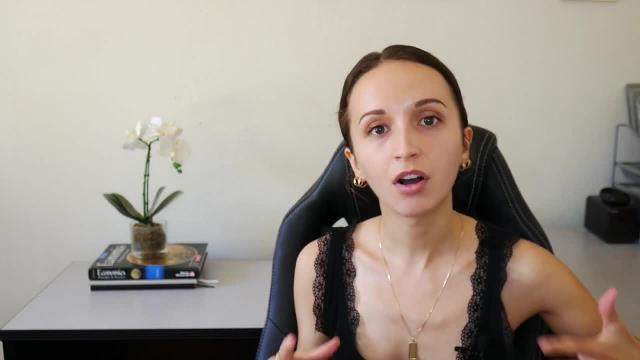 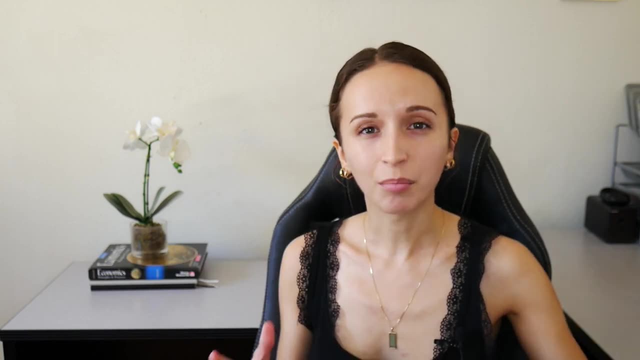 continue or terminate a business venture. sunk costs are completely ignored. They are held independent of the decision that has yet to be made. And the problem is, as everyday humans, sunk costs may be the only thing we account for when making a decision. 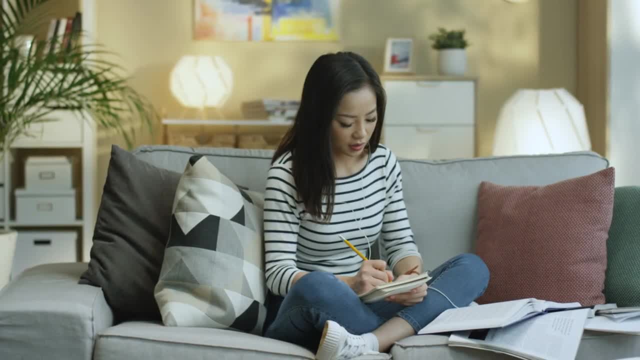 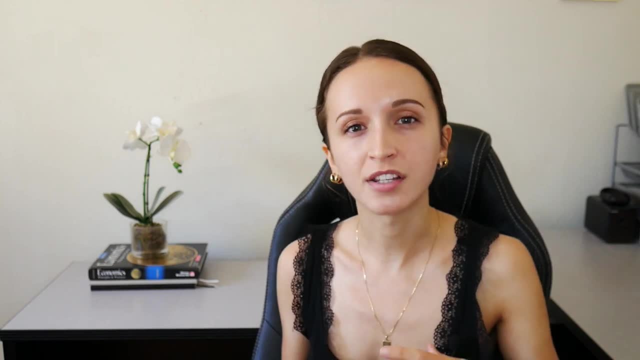 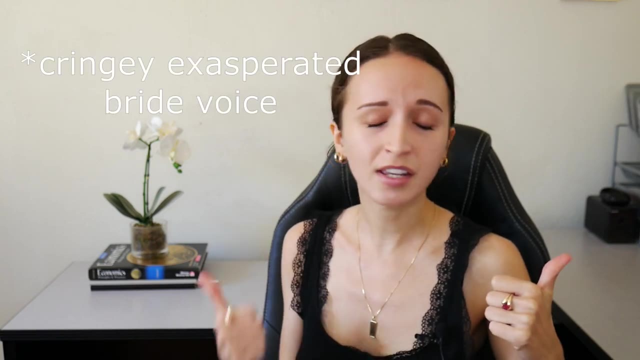 I'll give you an example of a woman planning her wedding. Let's say intuitively, she knows that this person is emotionally manipulative and toxic, but she rationalizes, moving forward with the wedding based purely on sunk costs. For instance, I've already spent six months planning the wedding. 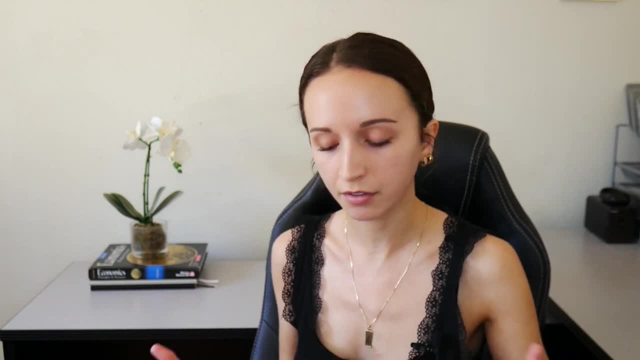 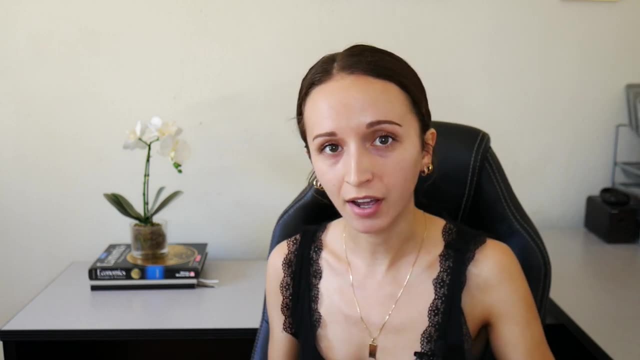 I've already put $10,000 for the venue and the catering. The invitations have already been sent out and people have already RSVP'd. And guess what? She marries the guy. She spends five more years in an abusive marriage that ends up ending in divorce anyways. 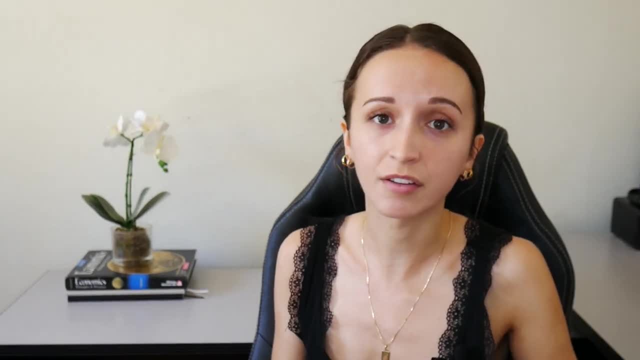 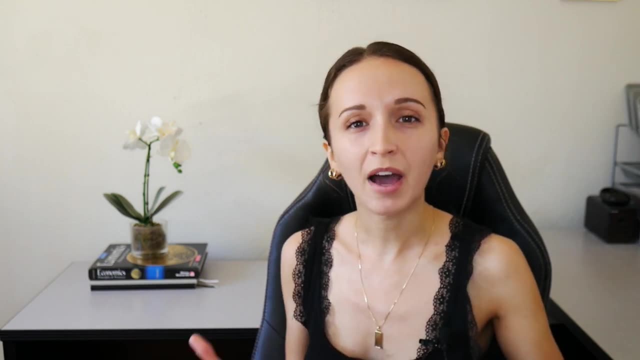 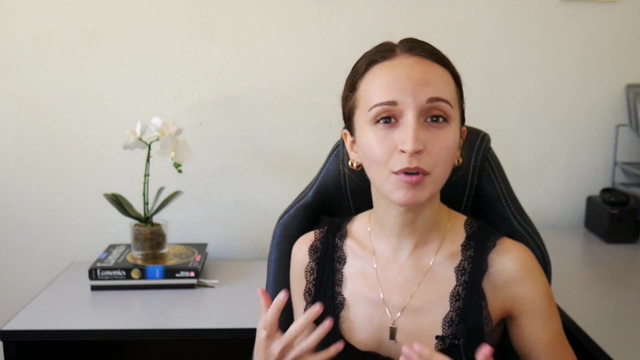 And, trust me, divorce is probably going to be way more expensive than that wedding you were planning. Don't be this person. You end up losing bigger later on and you have to backtrack on that decision later on. anyways, We are, by default, irrational, emotional and perhaps most crucially and to our own demise. 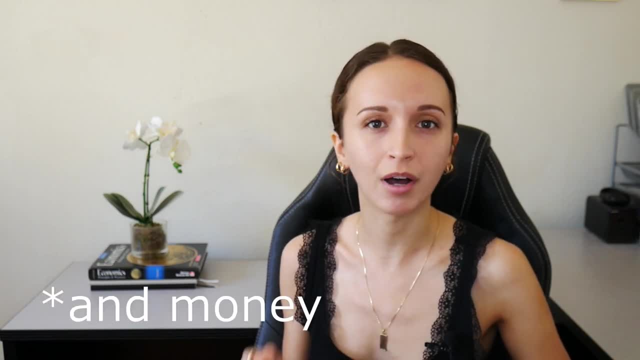 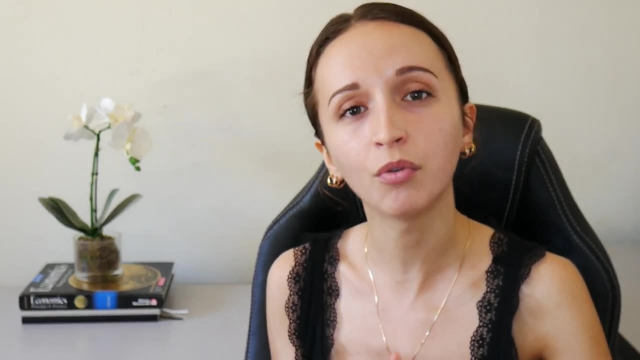 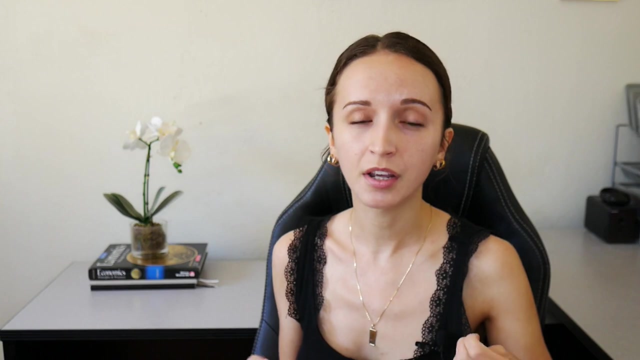 really, we prioritize conserving energy above all else And we ignore our intuition, based solely on sunk costs. Sunk costs should be ignored. This has been far too condensed of an explanation, but for the sake of time and engagement, I'm going to move forward to number two. 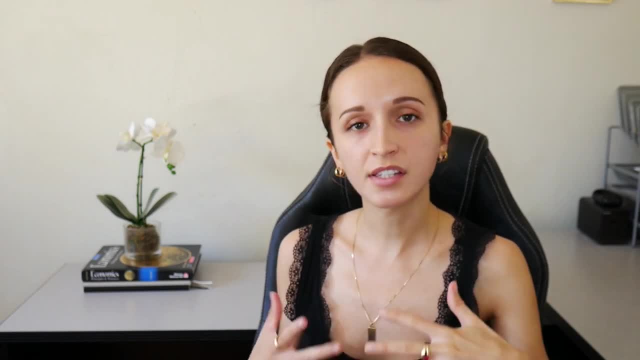 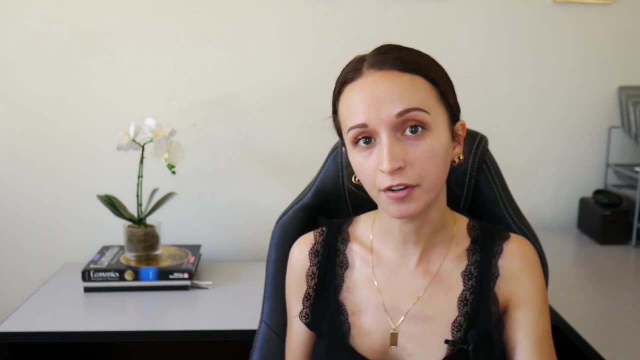 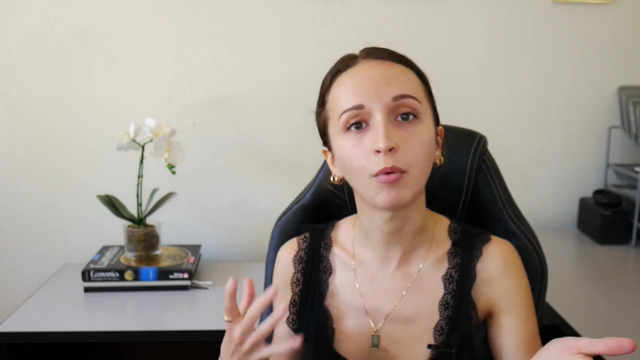 A cost benefit analysis is basically this systematic process in which you measure the benefits Minus the costs of a certain decision. In economics this is usually expressed in monetary units. If that resulting number is positive, benefits outweigh the costs. That means it might be a good idea to continue forward with that decision. 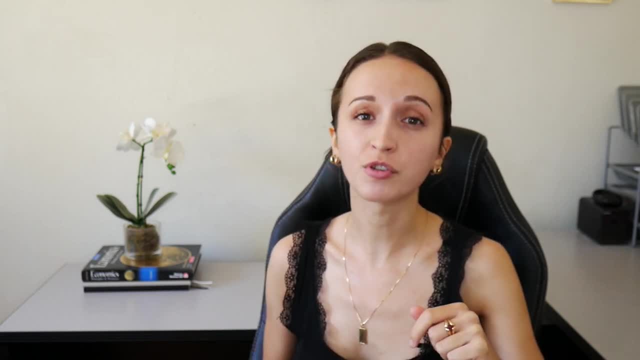 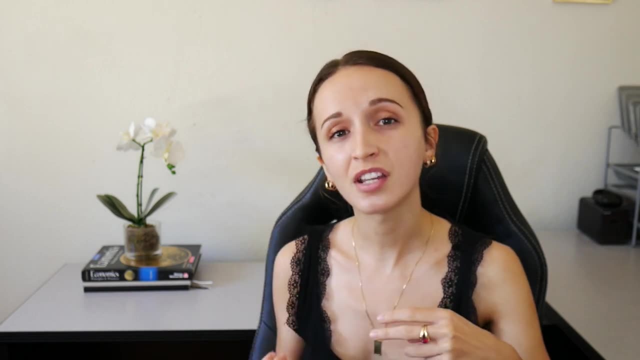 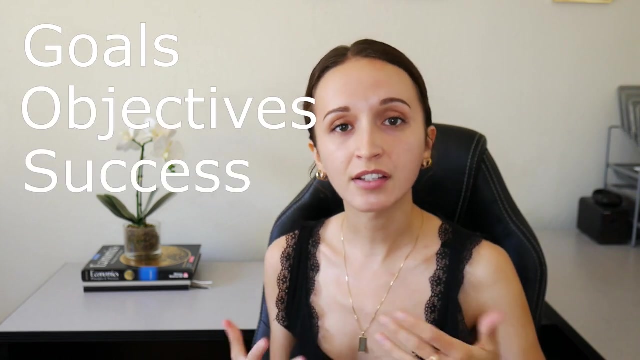 If it's negative, meaning costs outweigh benefits, it might be time to rethink that decision. A cost benefit analysis is pretty systematic and exhaustive by design. You have to sit down and really take some time to define your goals, Your goals and your objectives, your definition of success versus failure, and also carefully. 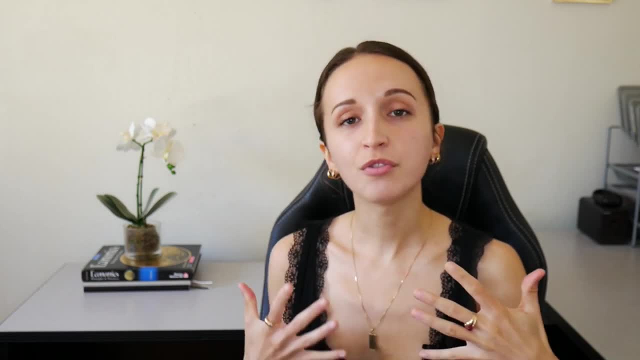 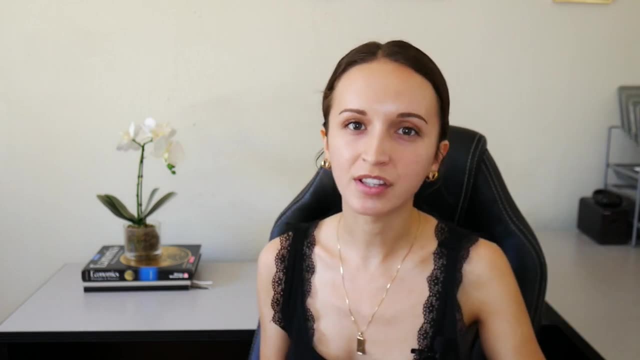 identify the costs and the benefits, Then you need to assign the value or weight to each cost and benefit. What I mean by that is, if you compare the costs and benefits of running a mile, you're not going to compare the benefit of increasing endorphins to the cost of becoming sweaty. 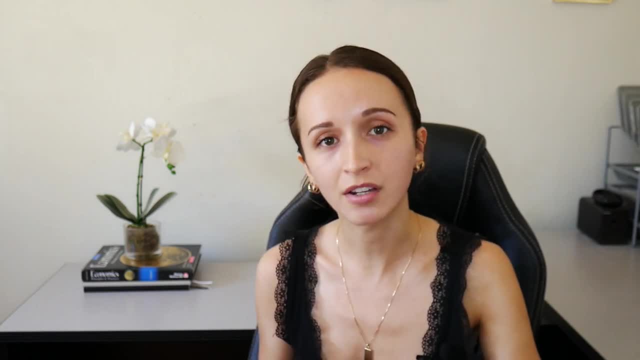 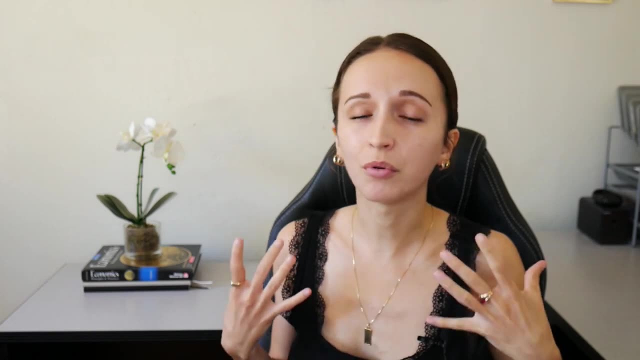 equally, because not all costs and benefits are created equal. That's what I mean by assigning value. Okay, So this is basically like a complex T chart. What is so great about it is it allows you to break down a decision into digestible components. 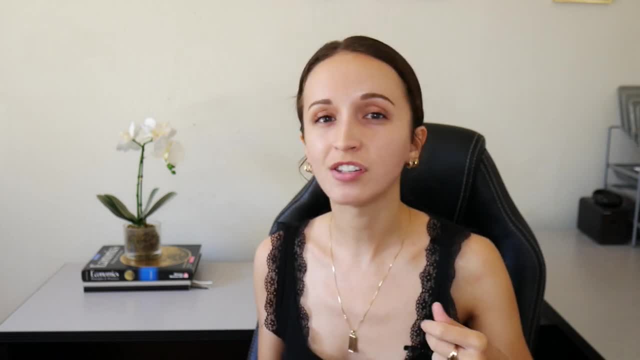 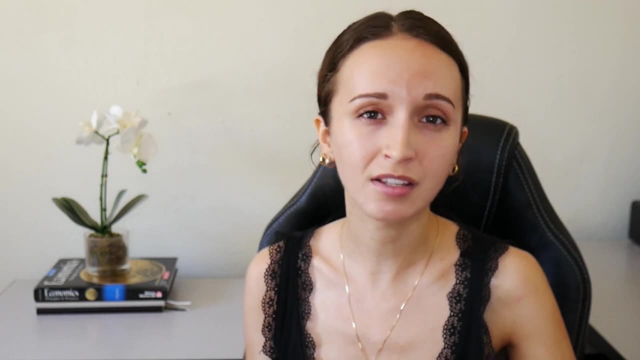 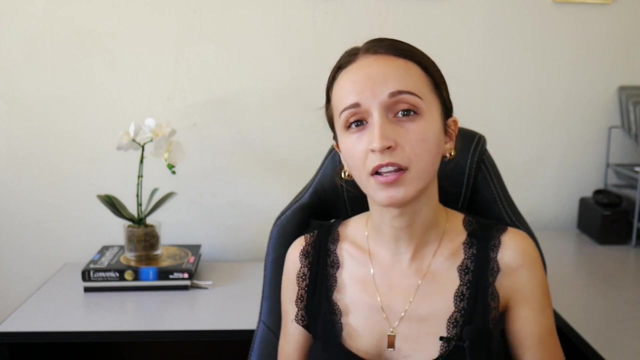 and define each component, which is great because it forces you to slow down and properly analyze everything, And I truly believe that people make some of the biggest mistakes when they make a major decision in a hurry, So this is great when you're feeling lost and need to redefine some important goals. 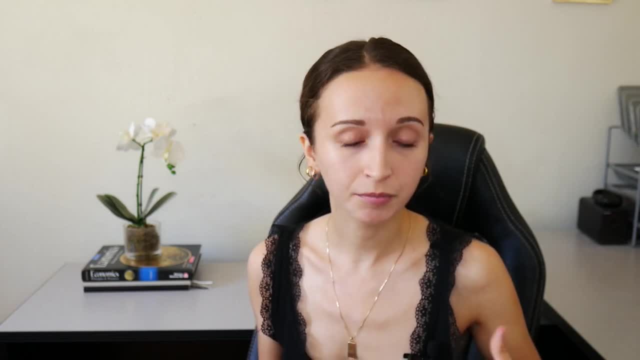 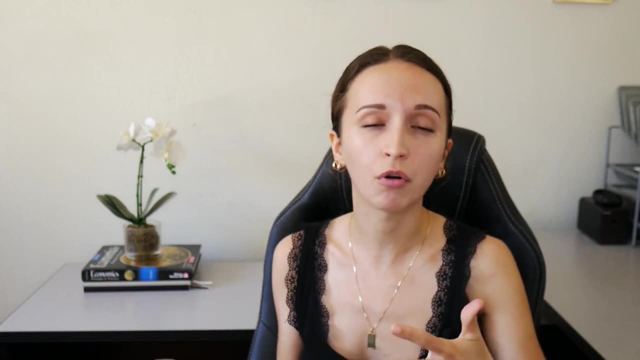 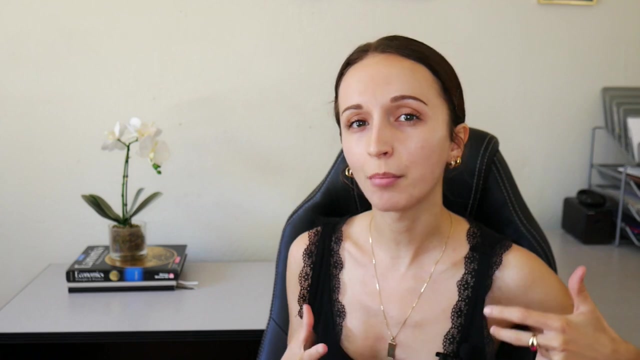 or life trajectories, But can't decide. Can't decide which road to take. So just create multiple cost benefit analyses for each possible decision you can make moving forward and then compare. Now, barrier to entry in the economic context refers to the factors that prevent or deter. 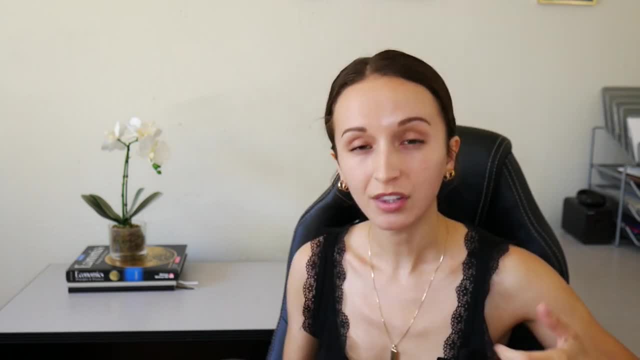 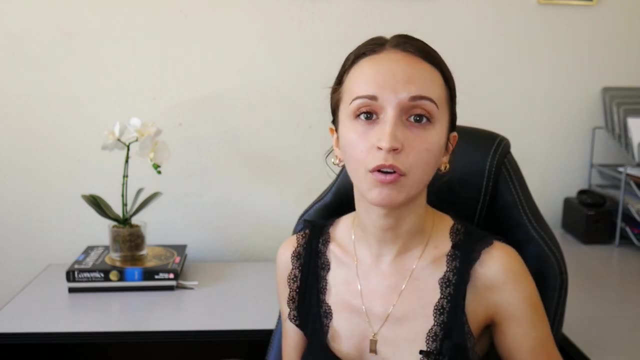 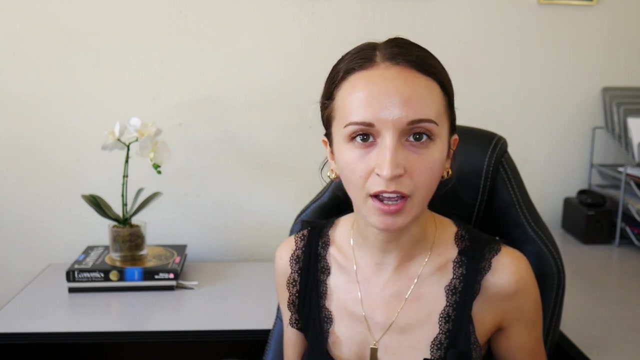 the entry of a newcomer into a market or industry. These factors are very specific to that particular industry, but can include things like high launching or startup costs, excess regulations. Now, this idea of barriers to entry pops up in many facets of everyday life, but most 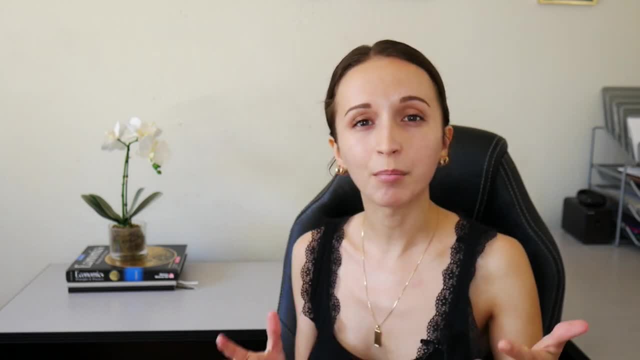 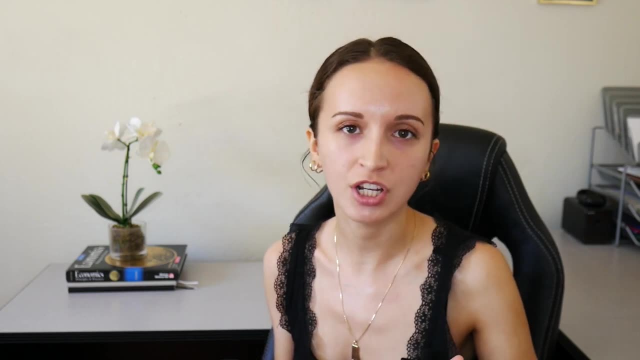 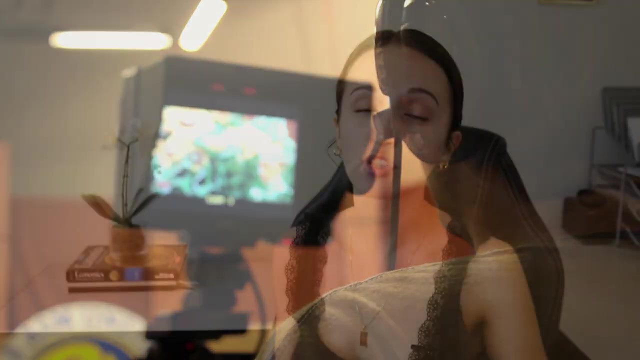 notably when taking on a new goal. For example, starting a YouTube channel has relatively high barriers to entry. It takes quite a bit of time and a hell of a lot of energy to even learn how to use the platform. learn how to film and edit a video and you likely have some startup costs for. 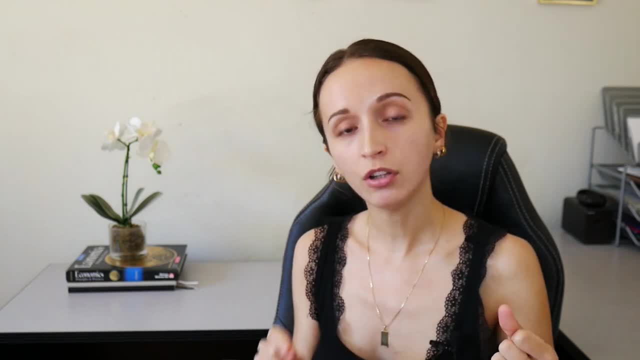 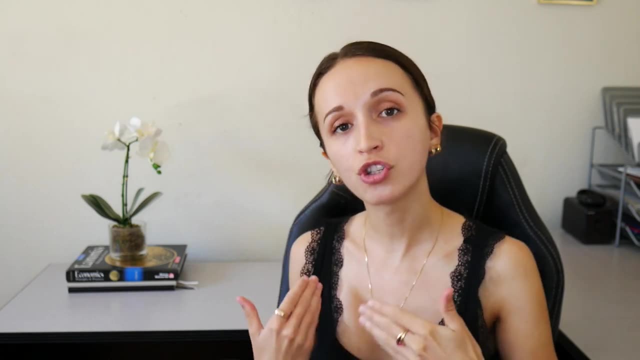 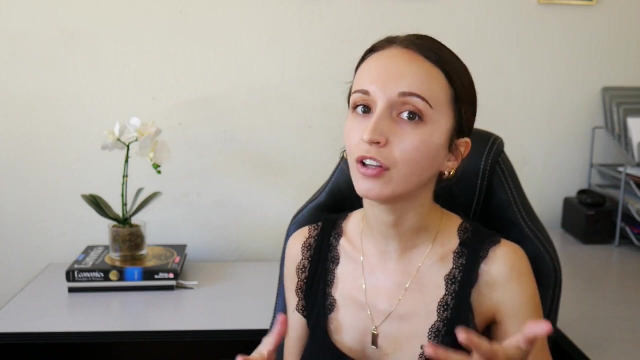 new equipment. So what's the bottom line? The bottom line: You need to look for ways to reduce your barriers to entry. In doing so, you increase the likelihood of you starting something that you've likely been putting off. So reducing your barriers to entry in the context of YouTube might look something like: 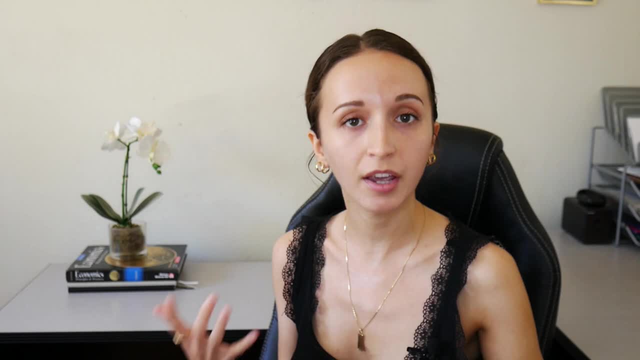 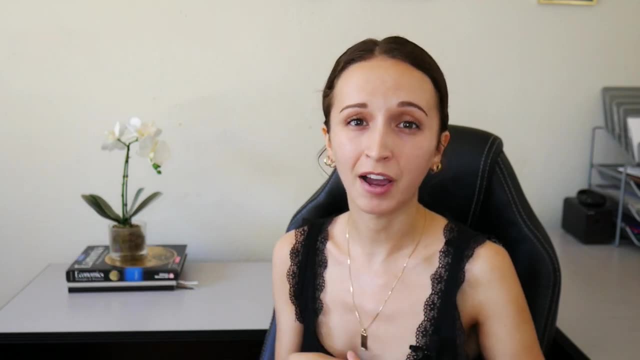 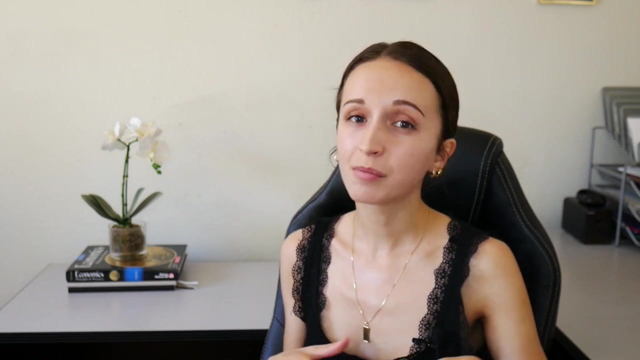 this Filming on your phone instead of buying a full blown camera. or buying a refurbished camera instead of a brand new one. Using natural window lighting instead of buying a whole lighting set. Or start filming. Or start filming smaller, less complex ideas so that you're not overwhelmed. 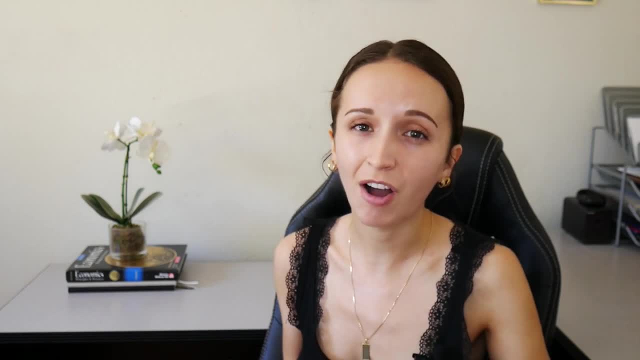 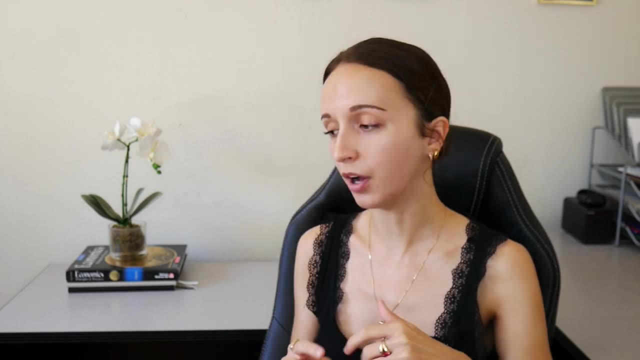 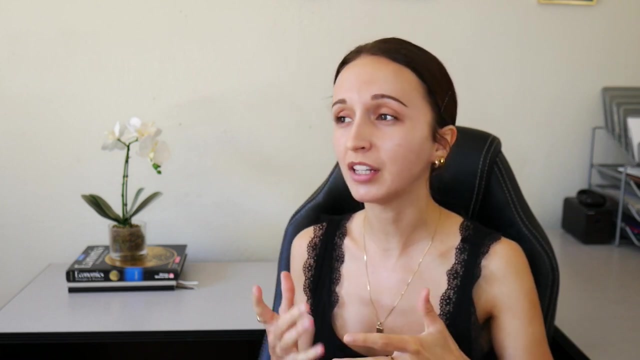 This might make you more likely to start your channel instead of putting it off for like another year. Also side note, I believe this can also help with reducing what I call goal resentment. We all have frustrations at the beginning stages of starting a new goal and I believe 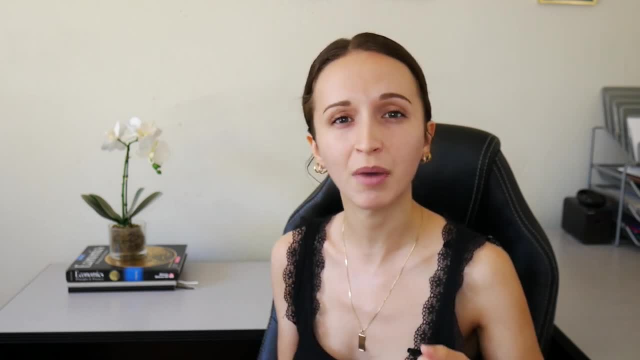 that if it's too frustrating and you have to sacrifice far too much upfront, you actually end up resenting that goal later on down the road. So if you're not able to do that, you're not going to be able to do it. 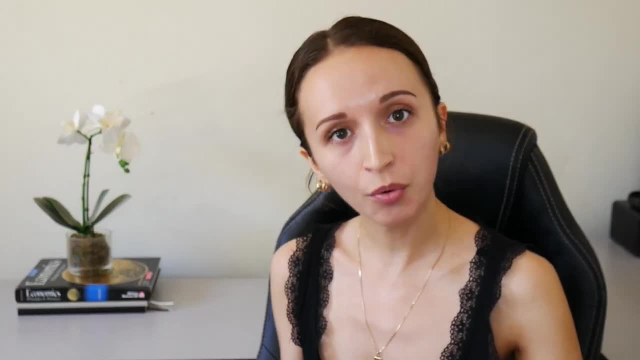 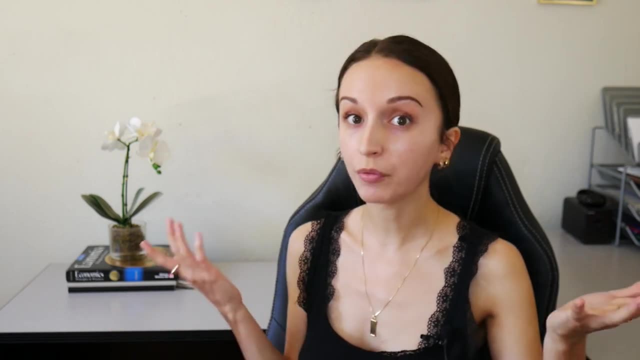 So if you're not able to do that, you're not going to be able to do it. This makes you more likely to quit later on. So reducing your barriers to entry can really help in reducing that goal. resentment, That's what I call it. 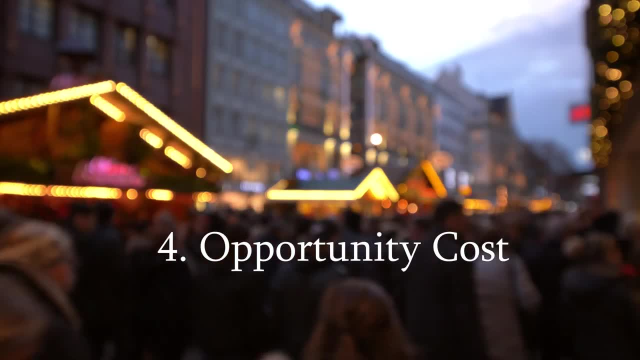 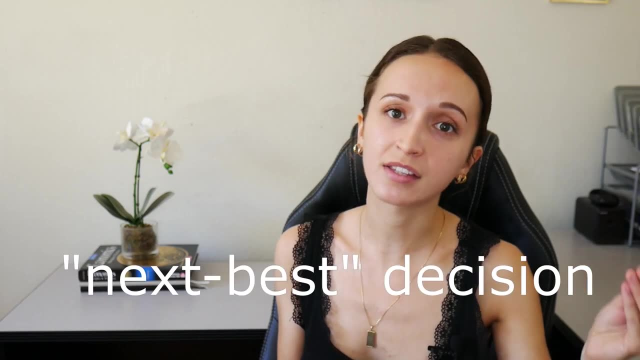 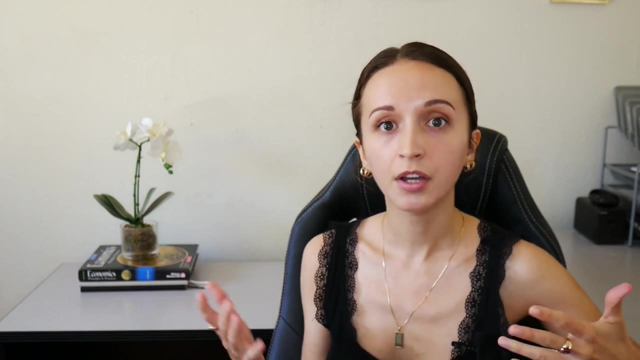 Win-win Opportunity cost is basically the cost that you incur when pursuing one decision over the next best decision. In other words, there's not only a cost to everything that we do as much as there is opportunity, But there's also an alternative to everything. 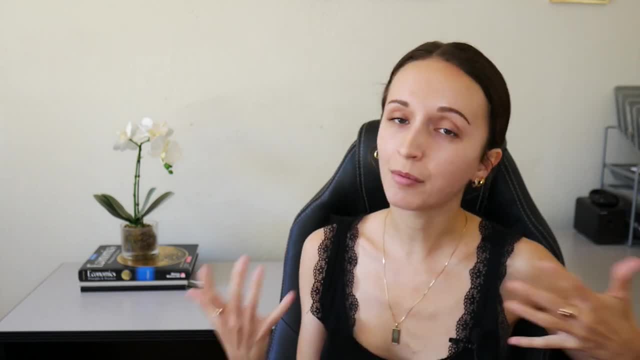 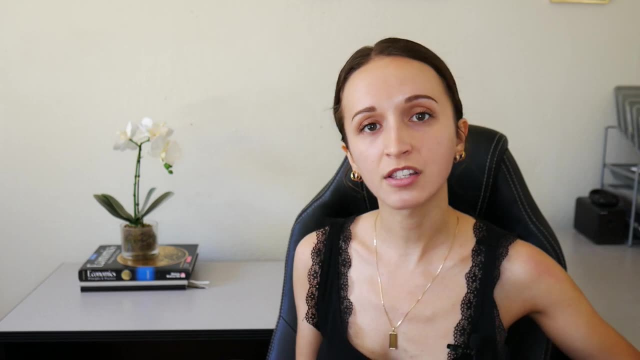 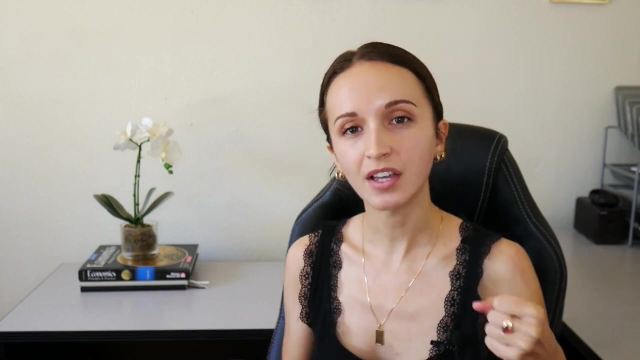 that we can do. Usually, our two most valuable resources, like I mentioned in the intro, are time and money, because they're limited, But it could also include things like enjoyment or satisfaction. So it's completely up to us how we choose to spend these resources, And you must think to yourself: is there? 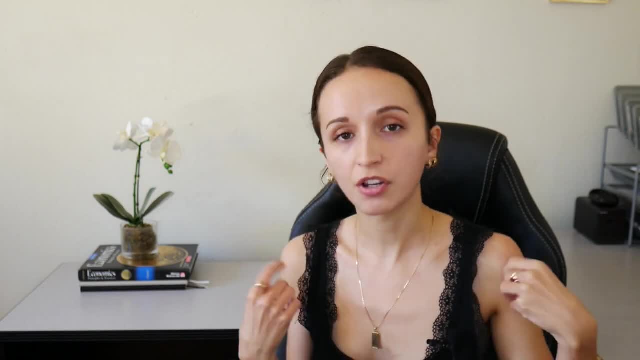 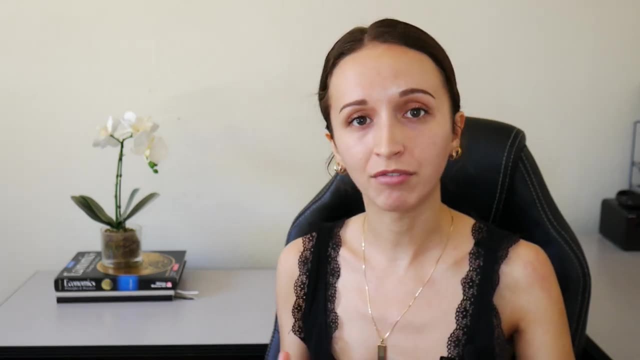 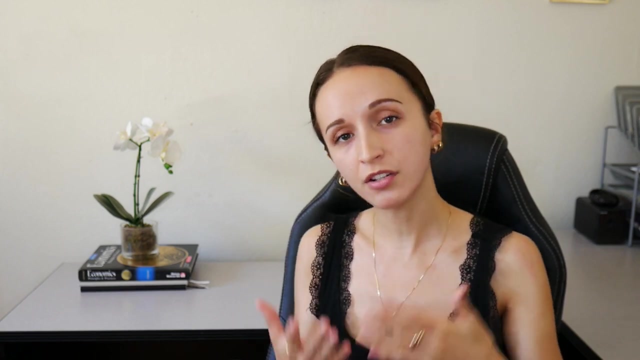 something better I can do with this time and money. So it really forces you, like a cost-benefit analysis, to analyze everything that you choose on a deeper level. Also, opportunity cost is subjective. The amount of time and money that you have available is unique to you and what you prefer to do with those. 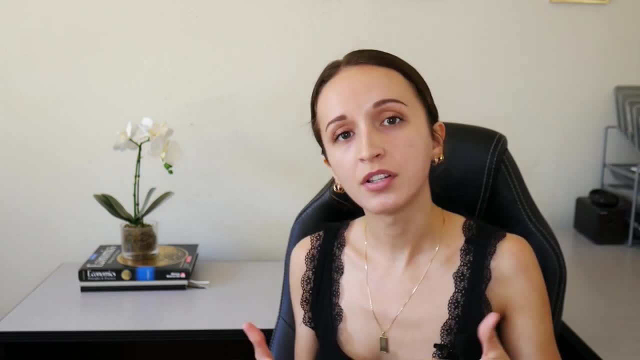 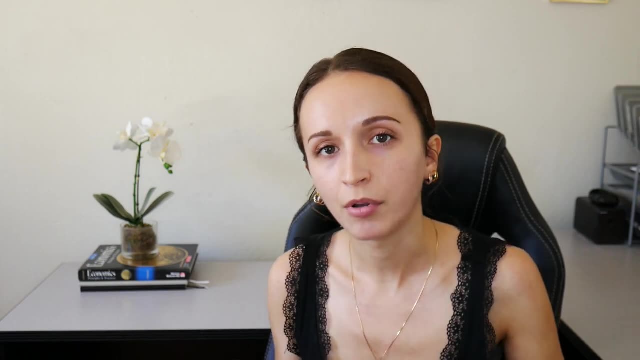 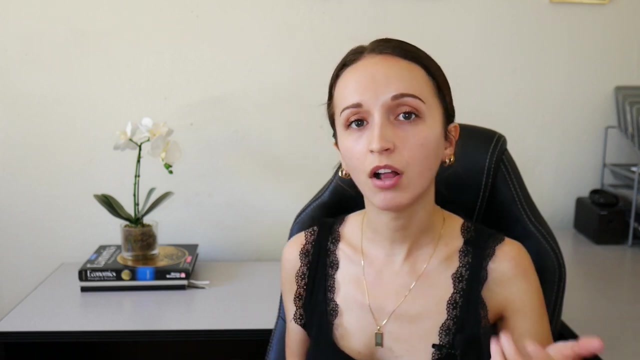 resources is also completely up to you. In other words, you have your own idea of what is considered the best decision and the next best decision. Take this common example of the opportunity cost of attending college versus working straight out of high school. full-time Attending college might be your best. 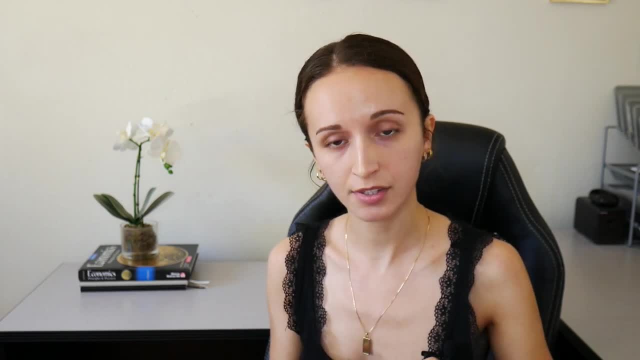 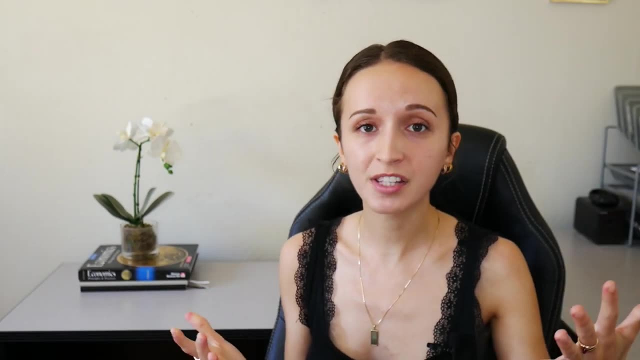 choice, While the opportunity cost of attending college might be your best choice. while the opportunity cost of attending college might be your best choice, while the latter is your next best choice, And the opportunity cost of going to college is huge and includes things like the tuition you're paying, which could be 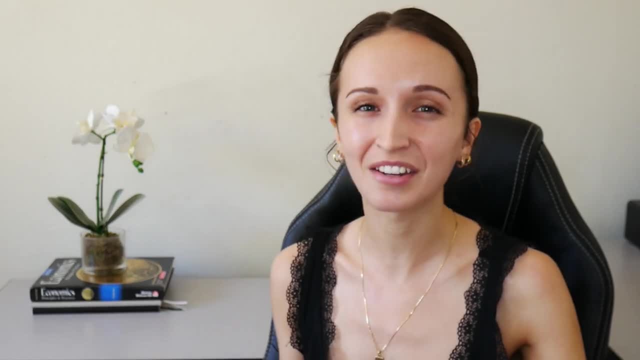 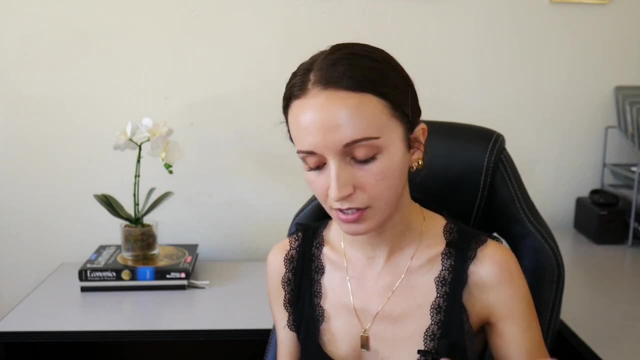 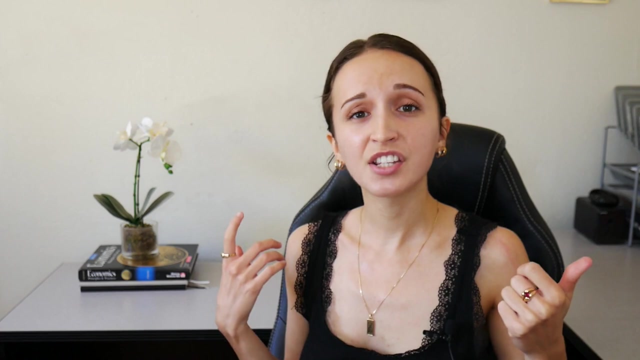 spent on something else, time and energy spent because college is not easy, as well as all the time you're losing that could be spent working towards financial independence. It's not just a question of what do I have to gain or lose by this decision. it's also a question of: is there? 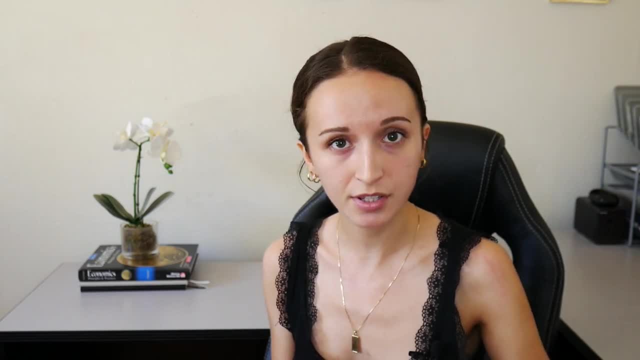 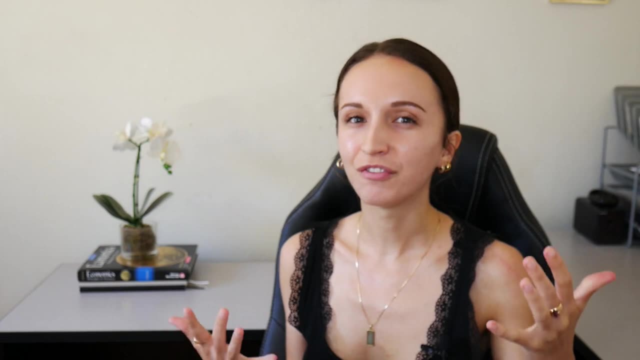 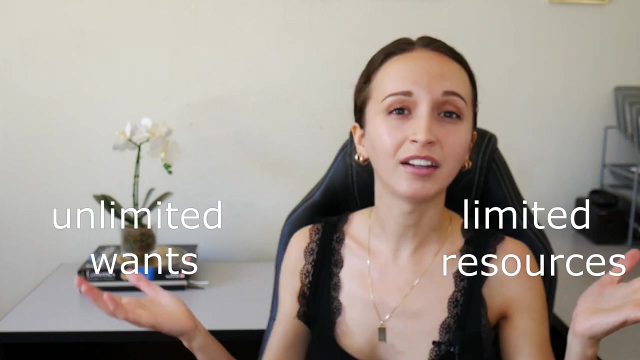 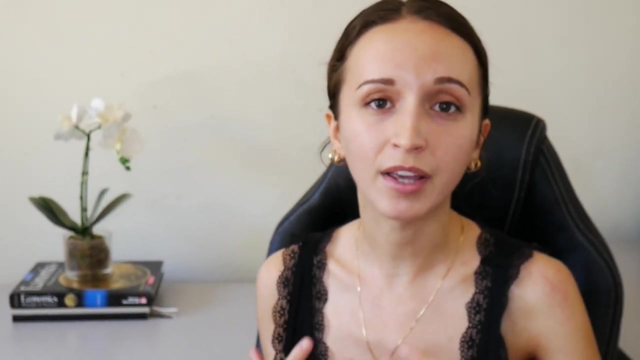 possibly a better alternative to using my limited resources, And it makes you think a little bit differently. Ah, scarcity, The fundamental problem that drives all economic study, The dreaded gap between limited resources and unlimited wants. No matter how productive we become, how much money we earn or how much time we think we have, we will never accomplish. 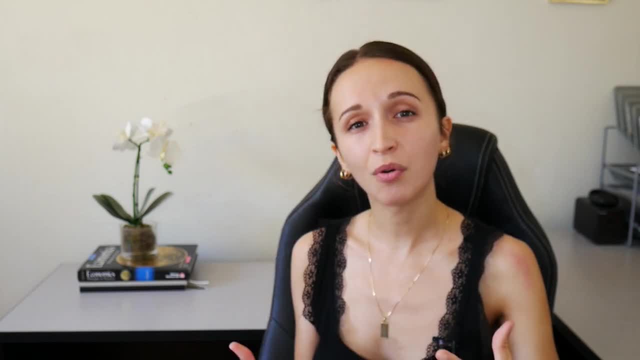 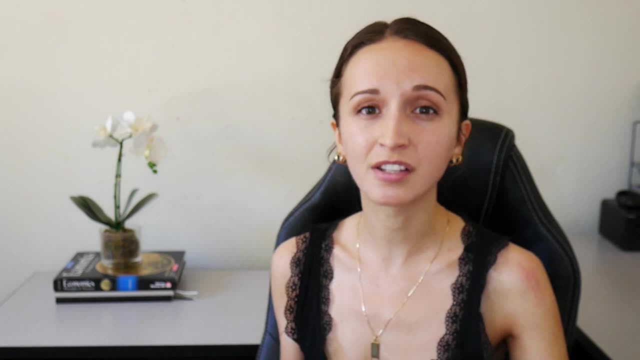 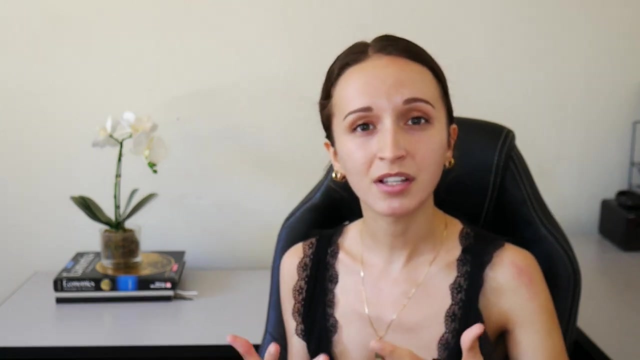 everything we want, buy everything we want or enjoy as much as we would like, Because money is not limitless, Time is not limitless And human energy is not limitless. Because of this idea of scarcity, we must face the dismal reality that there are limits. 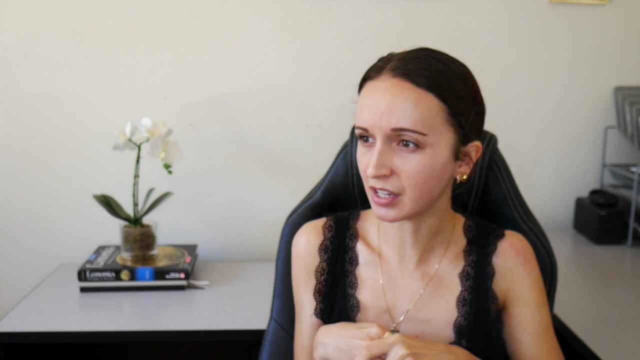 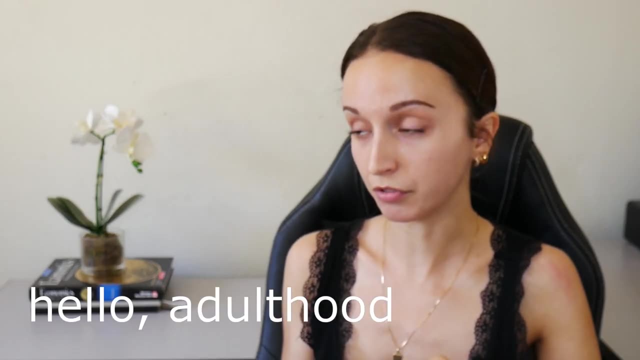 to what we can do. I guess the only thing that's limitless really is, well, the ability to desire more. Now, what's the take-home lesson from this? Well, adjust your expectations for one thing, But the other takeaway is this: Scarcity should. 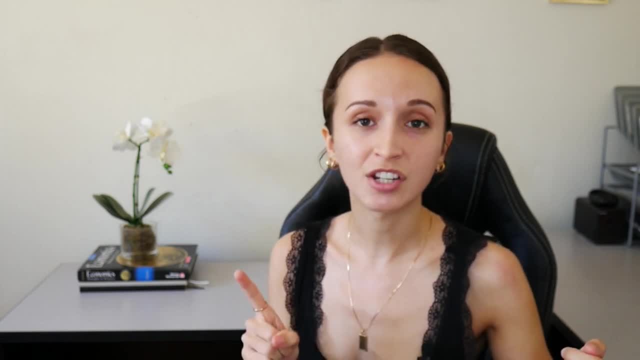 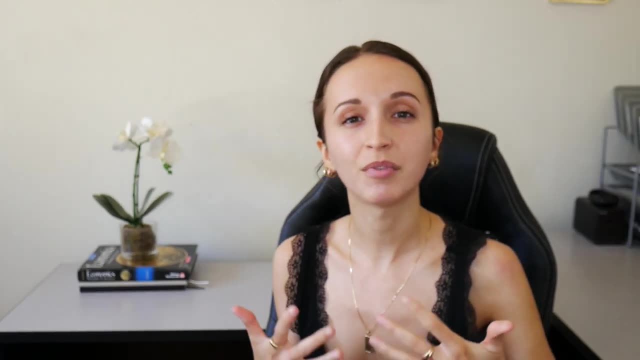 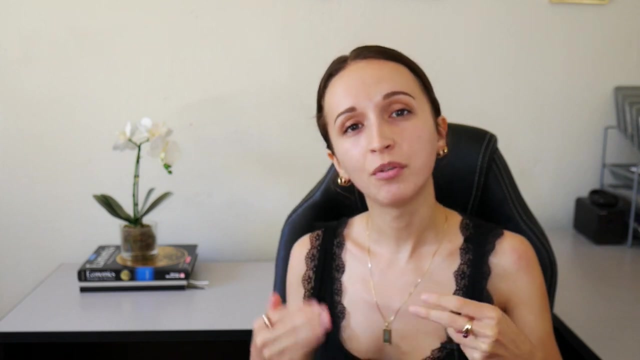 be the ultimate motivator, Not only for making better decisions in your your life, but also enjoying life as it is in the present moment. If we come to terms with the fact that money is a limited and incredibly important resource, we'll likely be more motivated to learn.